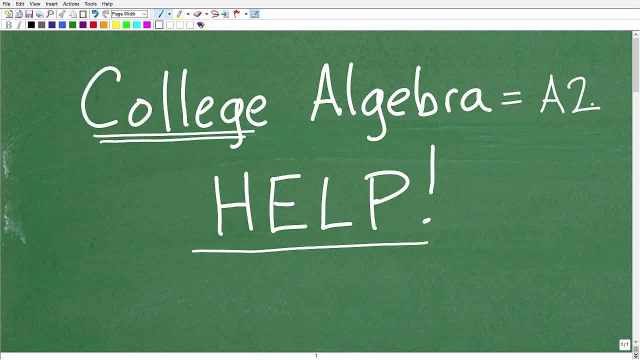 high school algebra, too, more or less Okay, but there are some distinct differences. So what I'm going to do in this video is give you some tips. If you're struggling in college algebra, that is going to help you out. Okay, but before we get started, let me go ahead and introduce myself. My name is John. I'm the founder of Tablet Class Math. I'm also a middle and high school math teacher And over the last several years, I've constructed many, many online math courses to include college algebra. So if you want to check out my full, complete college 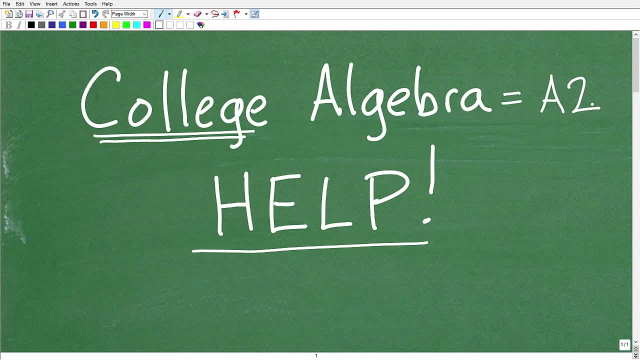 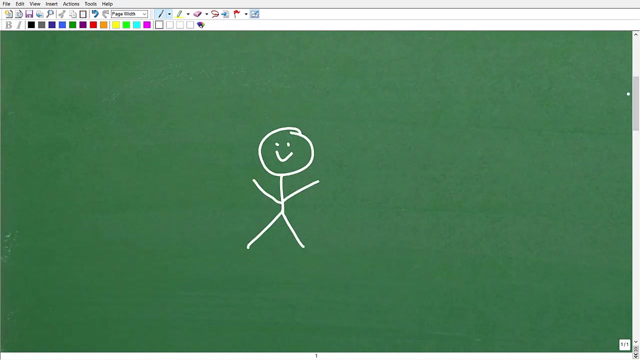 algebra course. I'm going to leave a link to that in the description of this video. It can really help you out as you get through your own college algebra. you know curriculum, But, with that being said, let's go ahead and get into how to get help with college algebra. All right, so a couple things here. Obviously, I mentioned that I have a full college algebra course- online course- But you know you're in. 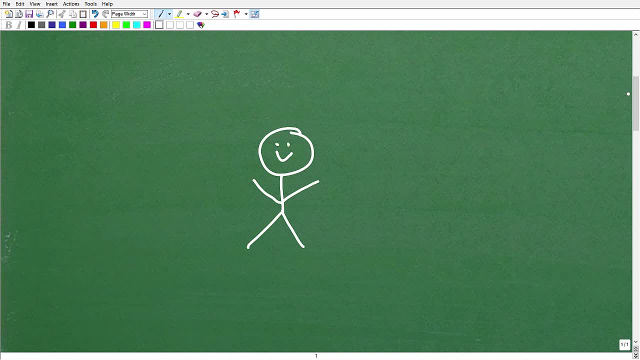 a course. right now You're out of school and you know there's a lot of pressure on you, right? So a couple things here. Let's just first quickly understand college algebra. So, like I said, college algebra, for the most part, is the same as high school algebra too, more or less. Okay, more or less Kind of think of it that way. So if you took high school algebra too- and most of you should have, being that you're, you know, taking college algebra- 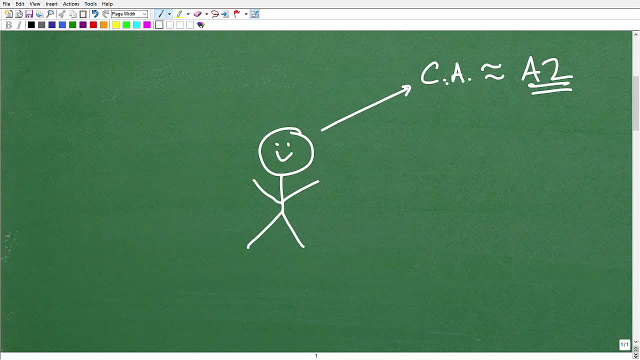 you know you're going to see a lot of those same topics, Okay, so the first thing is just know that you. you know this shouldn't be completely foreign to you, right? You're not talking about calculus or anything else along those lines, But here's a couple big differences. College algebra could tend to be a little bit more advanced. Okay, now, not every. every university's college algebra is going to be different from you know each other slightly, Okay, And everyone's high school algebra too. 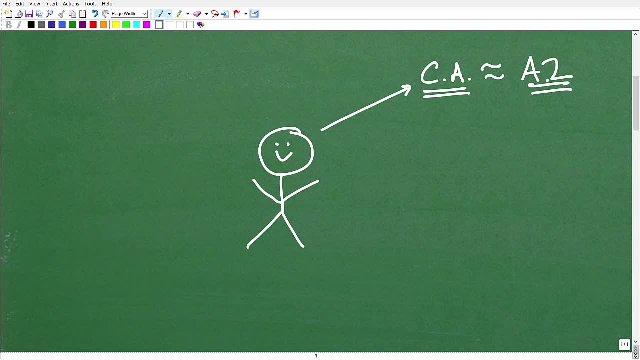 is going to be slightly different. So this is doesn't match up perfectly, But college algebra tends to be a little bit more complex than algebra two. This is the trends that I've seen through many years. Okay, The other kind of thing that makes this a big difference for most students out there is: in college algebra is generally a semester class, where algebra two in high school is a one year course. Okay, so you can kind of see what's going on here. 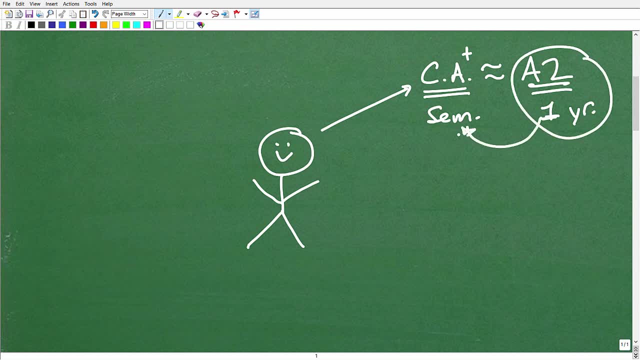 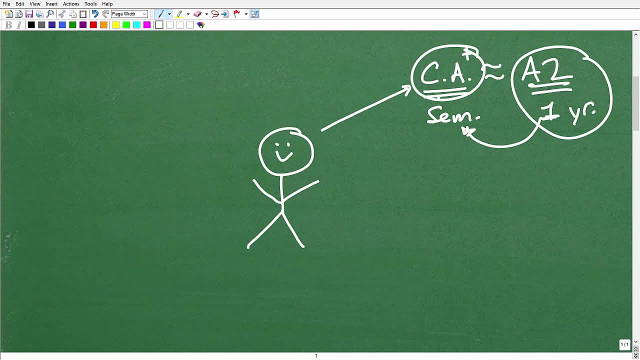 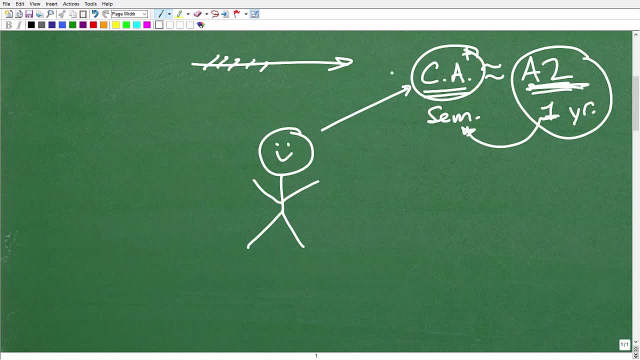 to get lost, okay. so this is a very common course where students struggle, and even even good students. okay, it doesn't make a difference. i know you're trying, you're doing everything you know, but maybe you feel like you're kind of drowning, so i just want to let you know that that's kind of a normal. 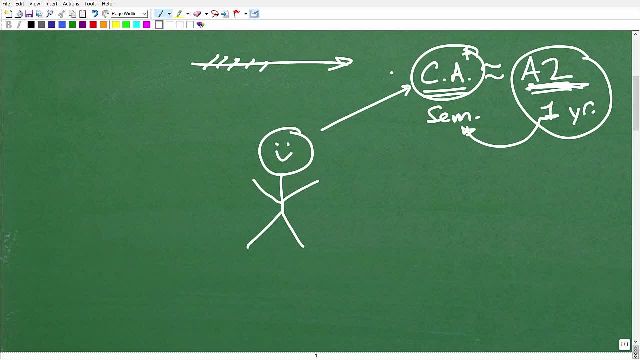 experience for a lot of students out there and- and i just wanted to give you some context on why that you know could be right- you're taking a year-long course. you're compressing it into semester. generally speaking, if you're taking college algebra for a full year, 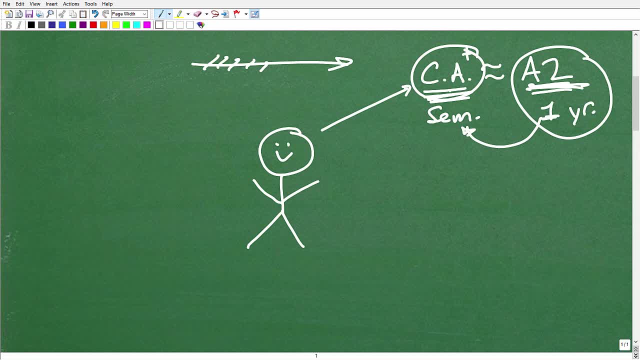 that's different, but most college other courses i've seen have been, uh, a semester long. okay, all right, so just a little context so we know what we're kind of talking about here. but let me erase this and now let's talk about what you need to do. okay, so the first thing is, uh, 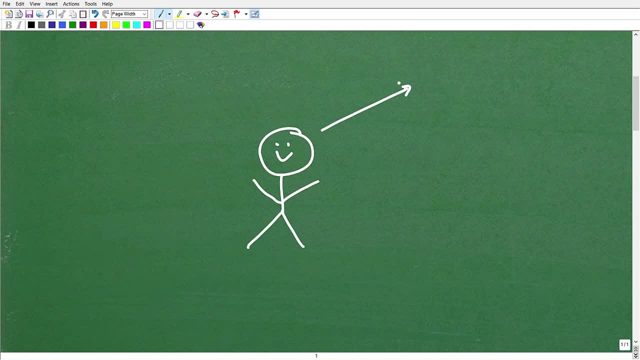 i always like to start. when you are- uh, or any student- taking a math class and they got a real student taking a math class and they got a real student taking a math class and they got a real challenge okay and you need help. the first thing is you got to check your mindset, okay. 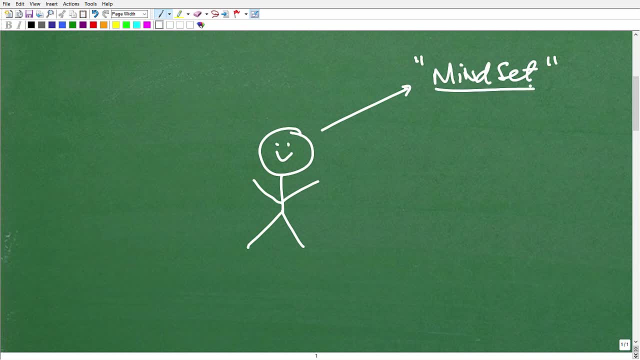 your mindset. your mindset has to be of one of like: okay, you have to make a determination right now. okay, especially early on in school year if you still have a lot of time remaining, and if you don't have a lot of time remaining, that's, that's. 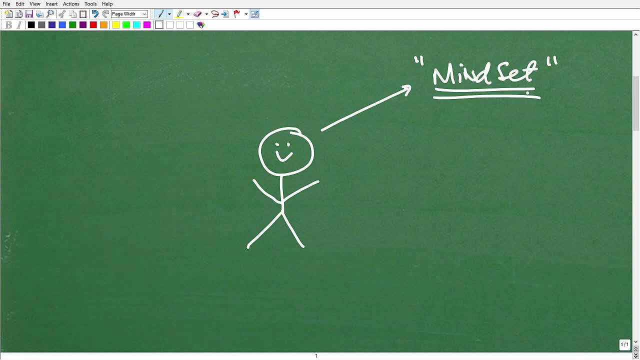 that's fine too, because your mindset is going to be the biggest thing that's going to help you. okay, it's going to start with you. okay, what thoughts are you putting into your brain? if it's more like i can't do this, i'm going to fail. 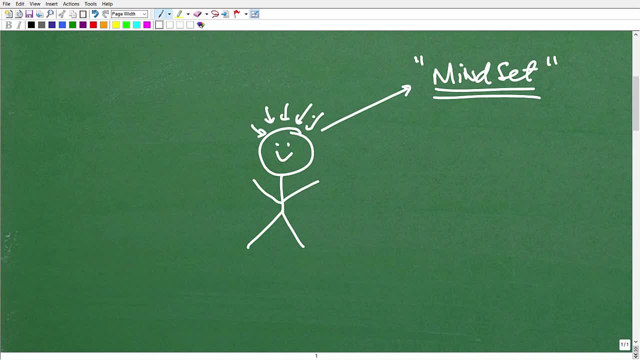 um, panicked, i can't. you know i'm struggling. no one's helping me. if this is your mindset, guess what? that's exactly what's going to happen. okay, you're not going to make it, so your mindset needs to be focused on. you know, solutions like i need to figure this out. you know i'm going to pass. 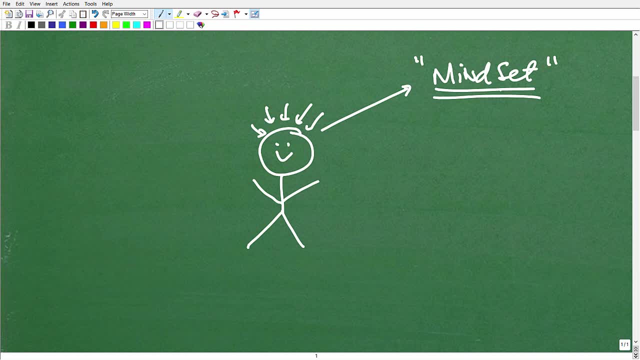 i'm going to do whatever it takes. so make sure your mindset, you know what you're thinking about. you know, in terms of college algebra, if you're struggling with it, you know, really, just commit to doing whatever you have to do to succeed. okay, and there are some real concrete things. 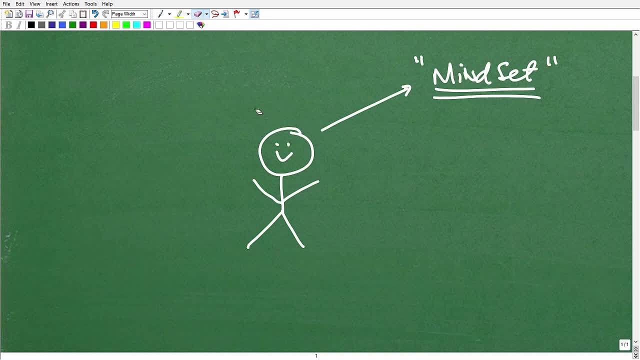 that you can do okay. so, first things first is your mindset, all right. second thing is going to be: uh, your teacher, all right, how much time are you spending with your teacher? right, you got to reach out to your instructor, all right, reach out. hey, i'm struggling. 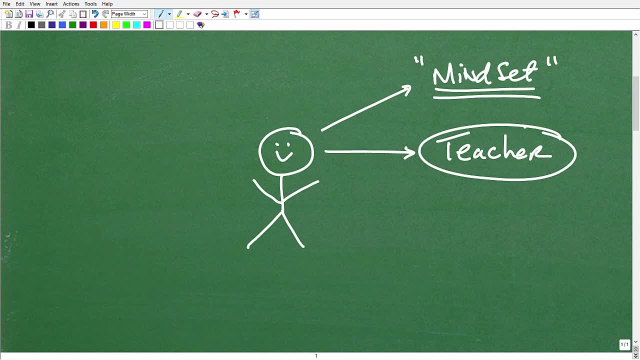 you know, uh, raise your hand. you know uh, email, whatever you know your situation, if you're doing distance learning and whatnot, so the, the. it should kind of go like this: the if you're doing you know poorly, if you're doing worse and worse and worse, right, if you're going down, down, down. 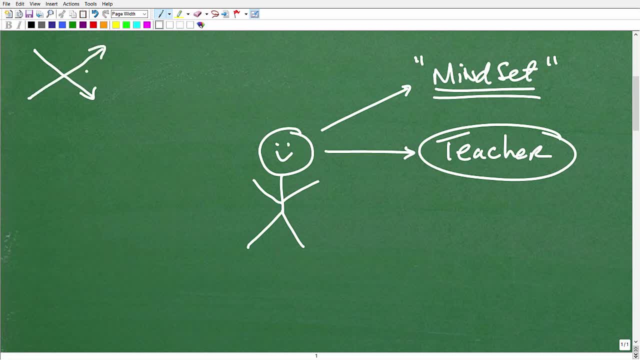 your time with your teacher should be going up and, up and up. okay, so that's kind of the deal. if you're doing great in the course, you're probably not spending much time with your teacher. if you're doing poorly, you know you're really struggling with the course. you should try to get as much. 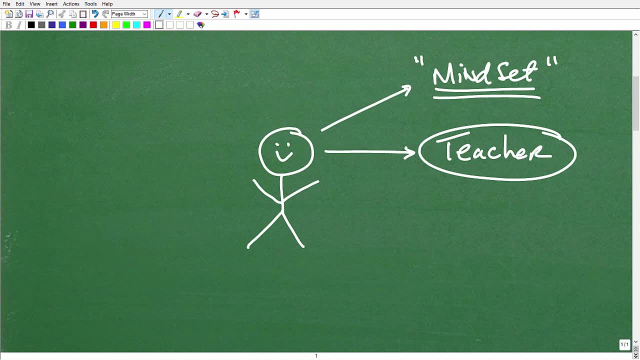 time as possible with your teacher and your instructor, an interest in you know, helping you. all right you're. they only got a limited amount of time, okay, and your instructor, believe me, wants to spend time, but those students that really need his or her help the most, okay, so reach out to your. 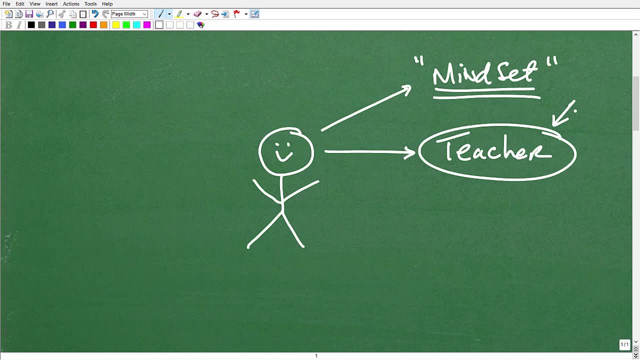 teacher. let them know they already know your grades. obviously they see what's going on, but you have to show initiative, that you care about passing. hey, what can I do? can you know? can I retake a quiz? look, here's a little trick. okay, I'm gonna give you a little inside tip about teachers. if a student asks a 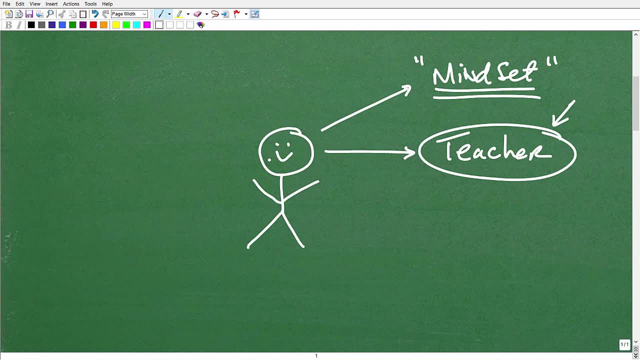 teacher. okay, can't like, let's say, you bombed a test or you really messed up a quiz. if you ask, even if the teacher doesn't invite it, but it just asked the teacher. hey, can I redo this test? can I make up some points on this quiz, can I? 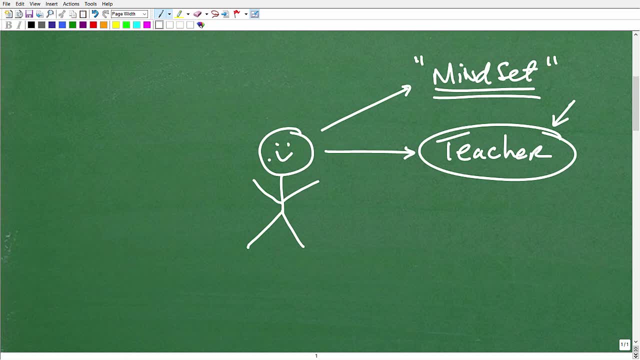 redo this? can I redo that, things that you don't think are their policy. just ask anyways, how can I raise my grade? what can I do here that? Let me tell you something. You pester a teacher, enough, a lot of teachers are going to give you ways, creative ways, kind of out-of-the-box kind of paths to increase your grade. 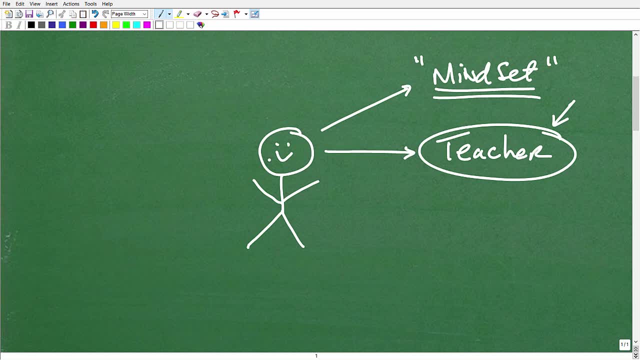 I've seen it from time to time. Again, not all the time It might just be marginally, but if you're persistent and you're actively seeking out assistance from your teacher one, you need to understand. hey, what's going on? I'm lost here. Can you show me this? Can I raise my grade, et cetera. 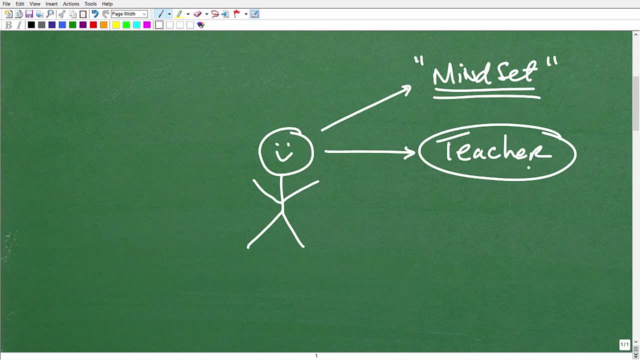 Make sure you're interacting with your teacher, because they're going to control your grade. They control everything, The two big things. when it comes to that, The next thing I would say is get into some sort of study group. So study group In other words, try to seek out. 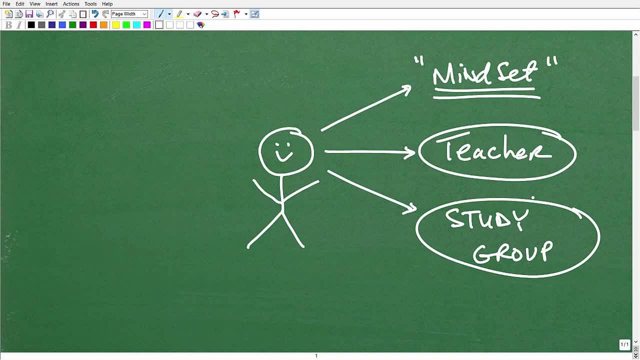 You know, students that you know are doing well, OK, and just kind of latch on to them if you can. OK. so you know, partner up with somebody who really you know. if you don't know, if you don't know of anyone, ask your teacher. 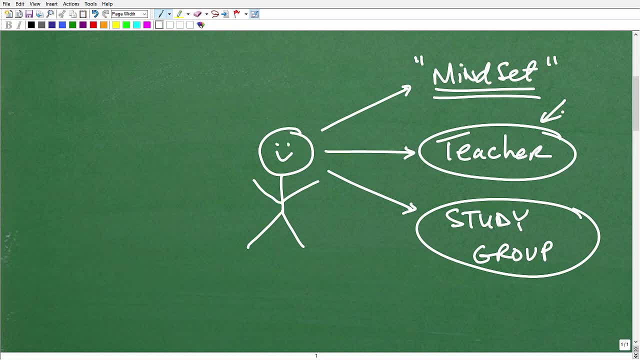 Hey, is there somebody you know in a class that you know is really good, that you think I might be able to work with or, you know, assist? Oftentimes your teacher will say, yeah, you know this person is doing really good You might want to see. 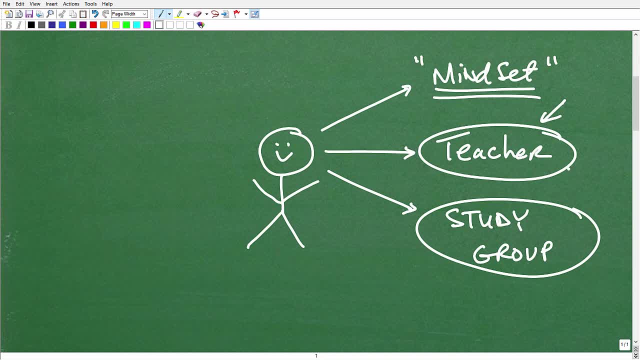 I'll talk to them and see if they can kind of help you out. There's all kinds of creative things, but you're not going to find out anything. This unless you ask questions. OK, so study group- try to find a study group. 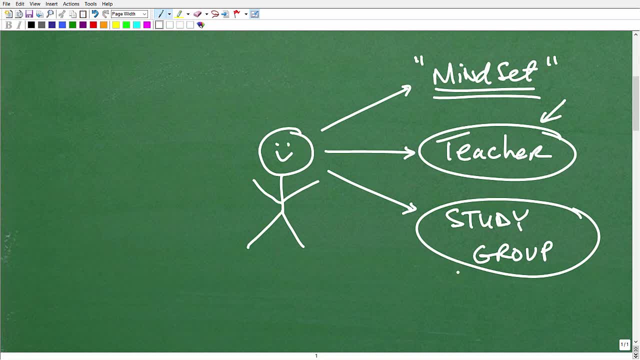 Now if you're at the physical campus, you know on your into a physical, you're going to a physical classroom with an actual teacher there. then it's going to be much easier to do. But seek out people who are doing well and try to see if you can kind of do your homework and study together. 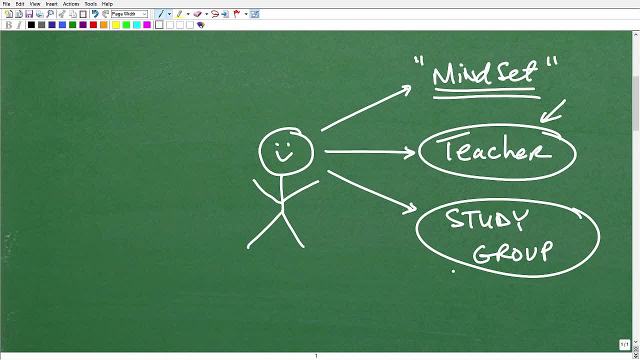 Don't be- you know, don't be- a solo artist if you will when it comes down to this. All right, So what are some of the things you can do? Well, you can use a supplemental program like mine. OK, so I have a tablet class math academy. 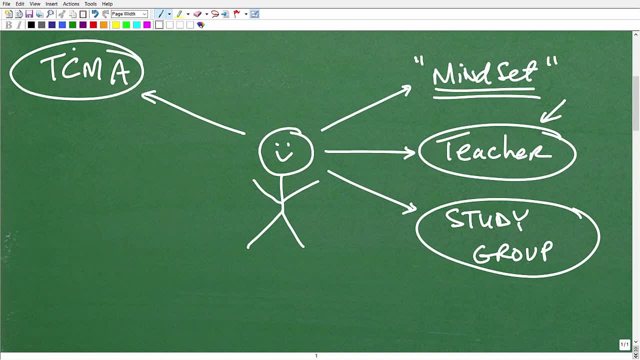 Now my program. I taught this course or it's complete, comprehensive, you know full on instruction, But you can use as a supplement. So for example, let's say your teacher is teaching about logarithms and things like that. 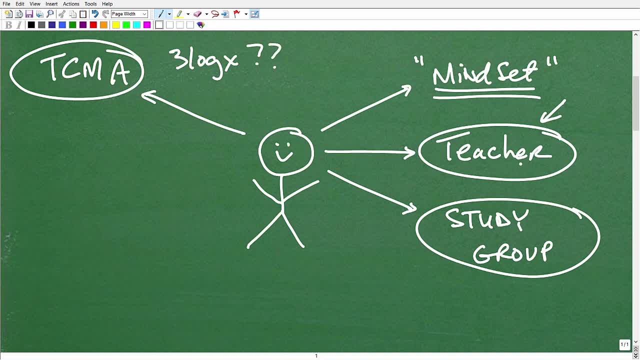 And you're just not getting it And you're like I don't get this. Obviously you're going to your teacher, You're trying to go to study group. But let's say you know you're going to a study group. 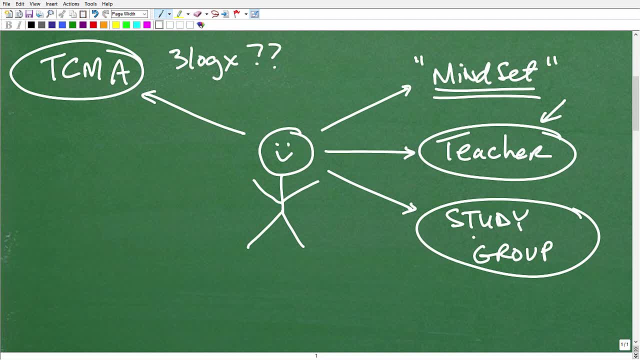 You know you're, you can't get into a study group because one doesn't exist, or your time, There's time conflict And maybe your teacher. you don't really quite understand them when they try to find kind of a supplemental, kind of tutorial type program online. 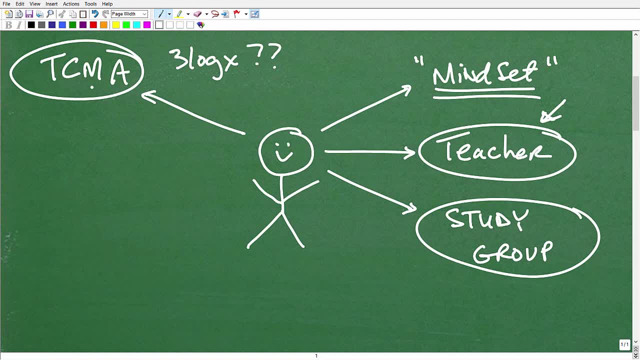 So like, the value of my program is you can go on there 24 seven and work at your leisure. OK, so kind of use it as a tutorial or complete full instruction, somewhat of a- I don't want to say a- replacement, But if your teacher is teaching about logarithms you don't get that, then you might want to find some other instruction to see if you can kind of connect the two. 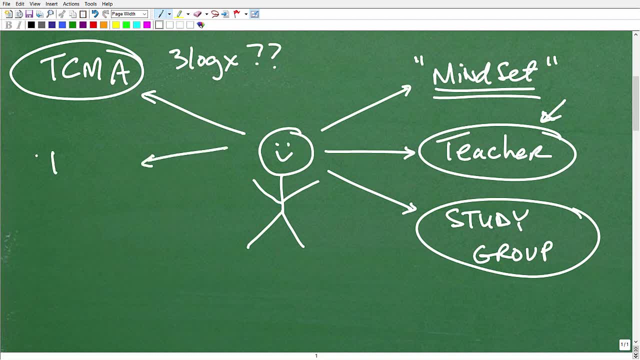 All right, OK, so another thing you could do is look for a tutor. OK, now tutors can be very, very expensive. Now how do you get tutors? Well, ask your teacher. See if there is a math center. OK, generally speaking, all colleges have some sort of math center. 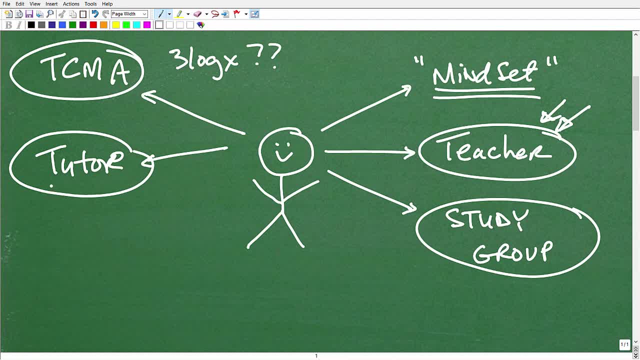 And then other might be graduate students or other college students that are really good in math that can act as a tutor. Oftentimes you could be free- at least for my university, You know- you can go into the math help center, sit down and some someone could help you out, et cetera. 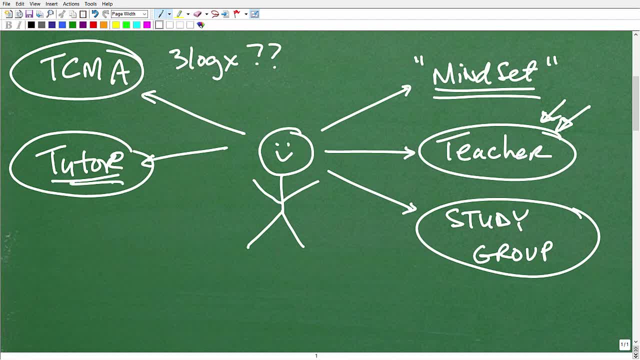 Or you can actually hire a another you know student who's really good at that and maybe you know pay. So yeah, you know you're going to have to make some investment sometimes, Sometimes. But if you need a tutor, you can. 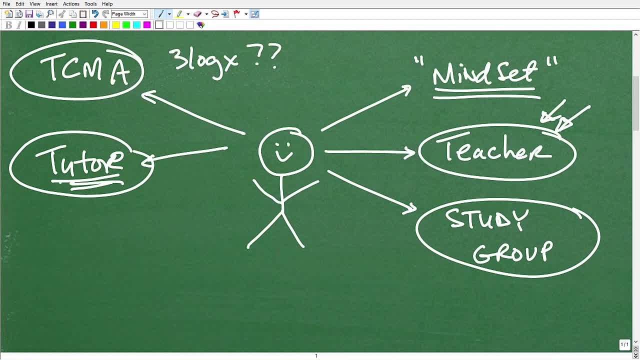 Get, they can be effective. But here's the problem with a tutor Right. One of the probably the biggest problem with the tutor All right Is: well, there's two things, OK. first of all, they are not, generally speaking, actual teachers themselves. 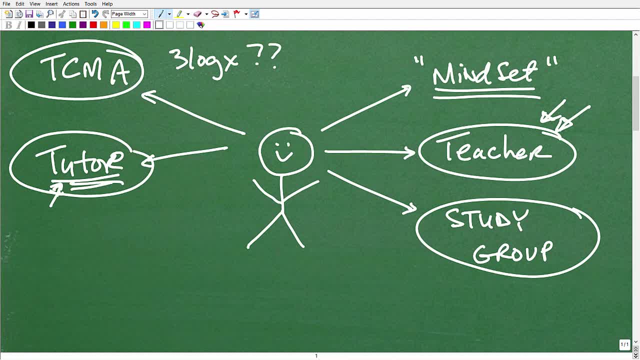 So there's students. although they're good in math, they may not be 100 percent on, you know, up to speed on all the topics. OK so, and that's not to say you shouldn't use them, but that's just kind of some of the things you need to be aware of. 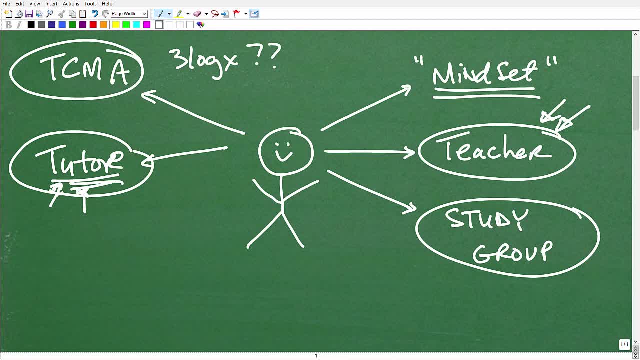 The second thing is: Is their scheduling Right? Sorry about that, Got to lost my frame of mind there for a second, But is scheduling Right? So you can only meet with them maybe in a half hour, an hour every other day? 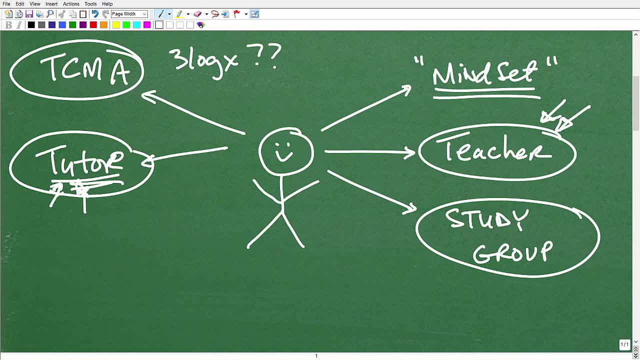 That's not going to be enough, OK, especially with the pace that your class is going. So some an online program where you can log in- you know 24 seven and stay on it as much as you like is more advantageous. You know a tutor. These are things that are options that were available. 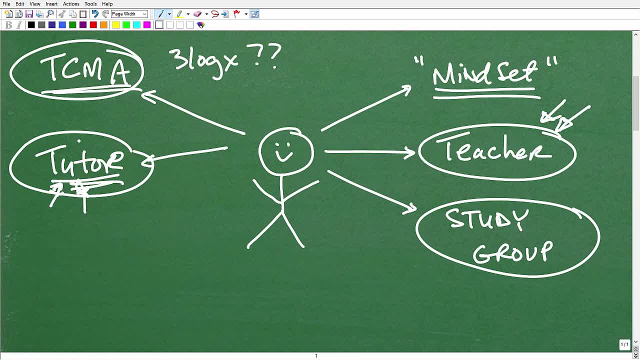 Only available to, let's say, students, you know, 20,, 30 plus years ago, because there was no online type of thing. But today there's a lot of things that you can- you can, you know, get assistance from from an online standpoint. 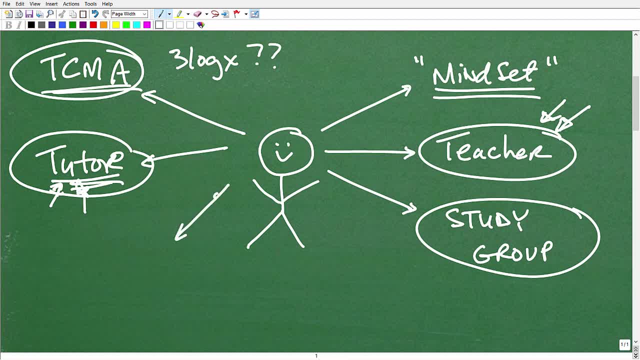 All right, A couple other things here real quick. Some real fundamental basic stuff that you should already know, But let's just kind of stress it anyways, is notes. How is your note taking? All right, Look at your notes and be honest with yourself. Are you doing the basic academic things Correct, OK, 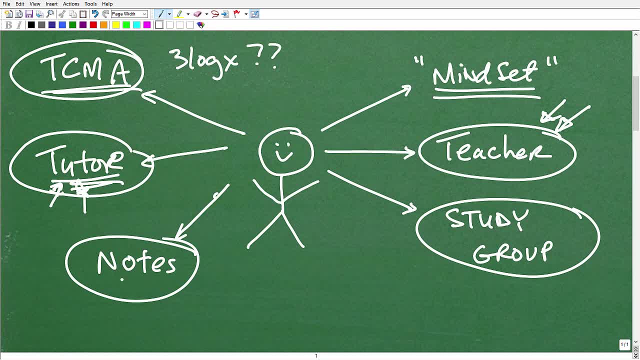 OK, Have good notes. Are your notes sloppy? Are your notes like? are you not taking notes? OK, Are you just kind of giving up? Your notes is probably one of the biggest primary indicators of how well you're going to do in a math class. 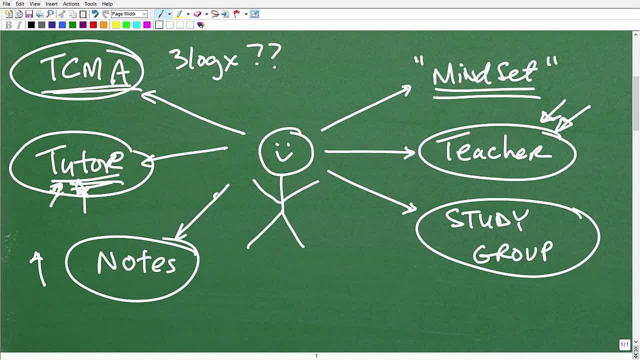 So increase your note taking in terms of how, how good your notes are Right. The better your notes are, the better your grade and your better your understanding is going to be OK. That's an absolute trend that I firmly believe as a math teacher for many, many years. 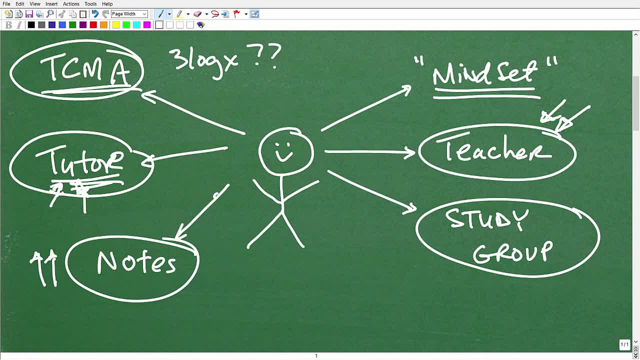 OK, So huge thing. And then a couple other things. here The obvious stuff is homework: OK. Make sure you do all the homework OK, And really put a lot of effort into it. If you don't understand you've got to go ask your teacher. 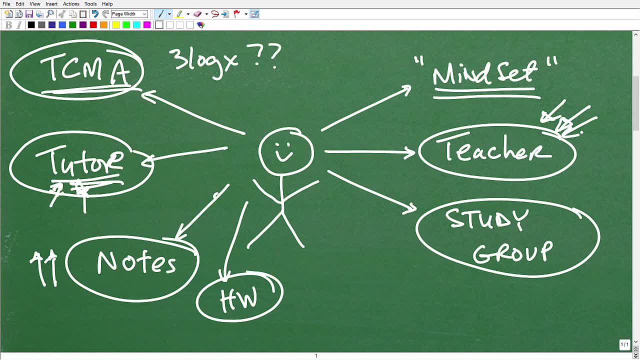 Hey, I don't understand this homework. I don't understand this, But you're not going to know what questions to ask if you aren't even doing the work, So you've got to be honest with yourself. OK, You've got to take a good look in the mirror here. 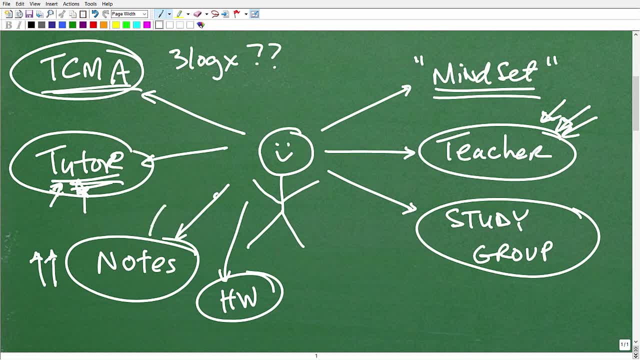 Like: are you working hard enough in this class? OK, Are you really engaged? Do you have great notes? Are you trying to do all the homework? This goes back to your mindset. OK, And if you're not working, if you're working hard but you can work harder, then you need to work harder in this class. 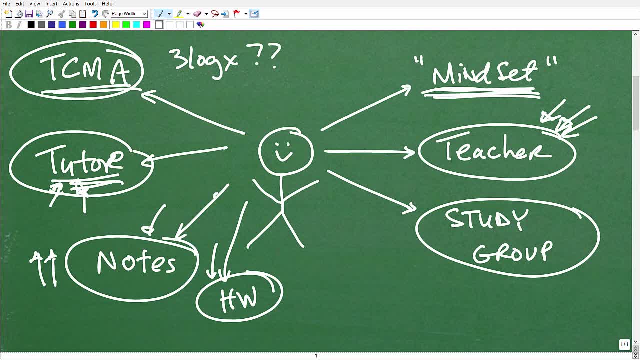 You're taking it out, You're taking a college level course. OK, You know you're going to have to do what you have to do to pass. This is in high school, It's not middle school. You're paying money for this. 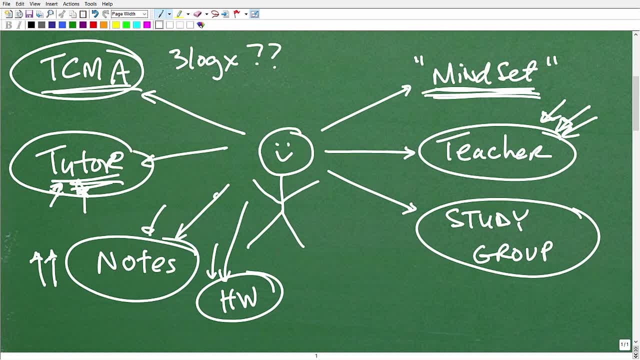 Your grades count. This is, you know, your investment in your education, Your education, your career. So you've got to do what you have to do, Right. So if you're working hard, that's good, But you need to work even harder, OK. 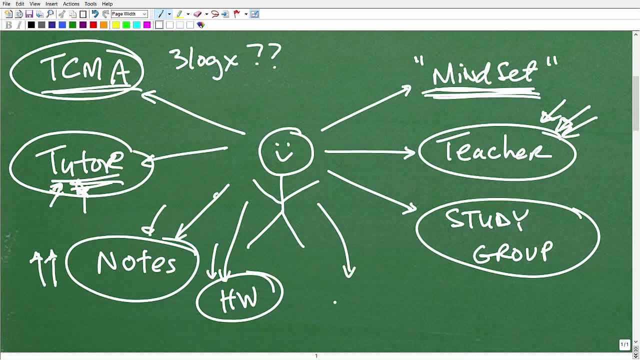 So notes, homework. So then, basically, when it comes to quizzes and tests, All right, You've got to be fanatical about that. Pay attention to the teacher. Ask questions again. What do we have a quiz coming up or what's going to be on a test? 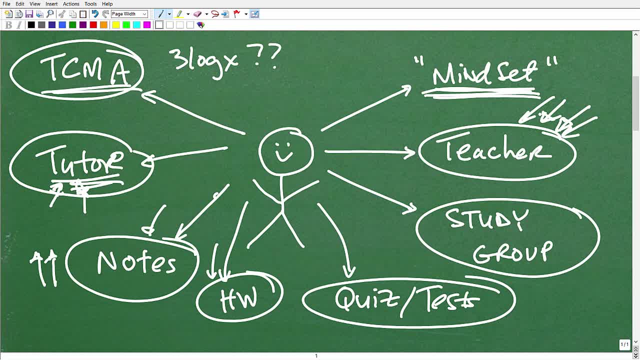 Do you think I do, I should, I, you know, you know, do my notes look good? I mean, you know, You have to be that, that student that just pesters your teacher. I'm telling you, I had those students that come to me. What about this, What about that? 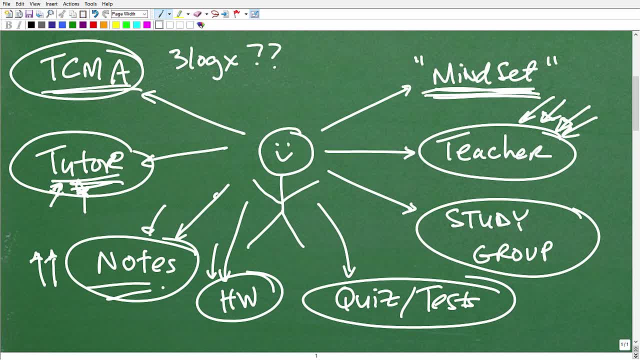 What about this? I'm like boy, this person just always asking questions. But guess what? I always gave them information Right, And oftentimes, you know, I try to share this information with the rest of the class. But they even asked more questions And it's almost like an intelligence gathering mission on things. 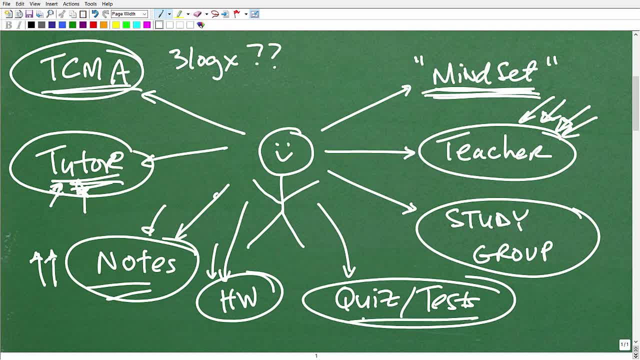 You'll be surprised that you can really- you know- find out much more about what's going on. Or you know how to prepare for a test quiz, just by you know asking questions to a teacher. Now here's one last point. We're going to wrap up this video here in a second. 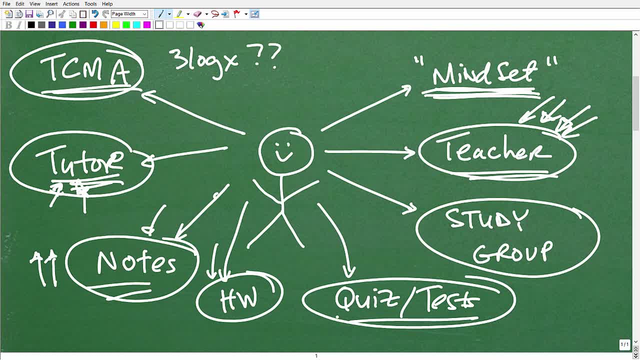 When you're, when all the dust is settled and you get some sort of quiz grade or test grade or final exam grade or whatever the case is, and you're right on the edge. Right, Let's say, your score is seventy eight point nine percent. 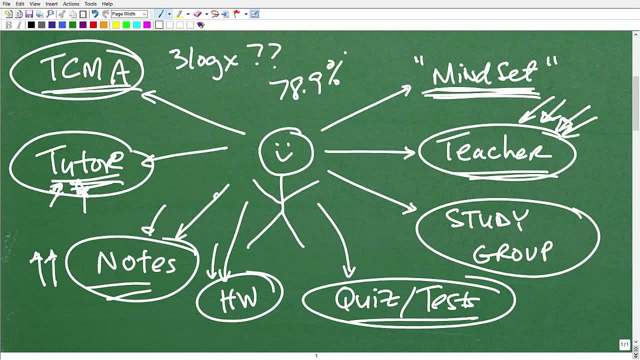 A teacher will look at your effort. How did this person, you know, you know, approach this course? Were they serious? Did they give it their best? You know, oftentimes a teacher will you know. I'm not implying that teachers cheat, but they do have a way of massaging the numbers. 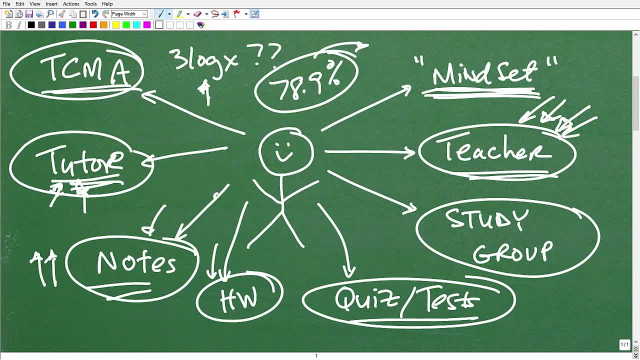 OK, maybe giving you a little bit more point value value on a particular question, maybe taking a little bit less off another question, because they know that, hey look, this is seventy nine. If they could get you to an 80 percent of B minus versus. 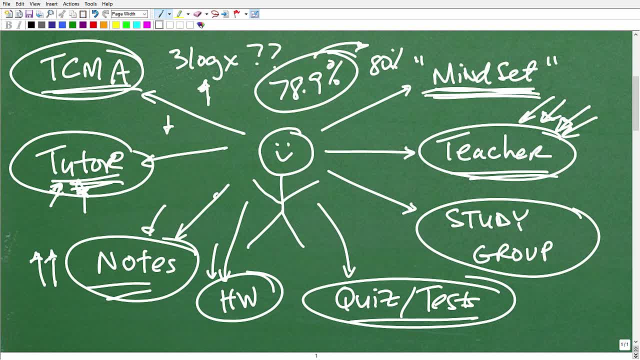 A, C plus. they realize the impact this is going to have. but they're not going to do this for all students. OK, they're going to go look to see what they can do, Take the extra mile in your situation. If you've showed that, if you take in our class seriously and you did everything you could, OK, you're going to set yourself up for the best chances of your teacher having, like a better word, some mercy on on you when it comes to, you know, being really close. 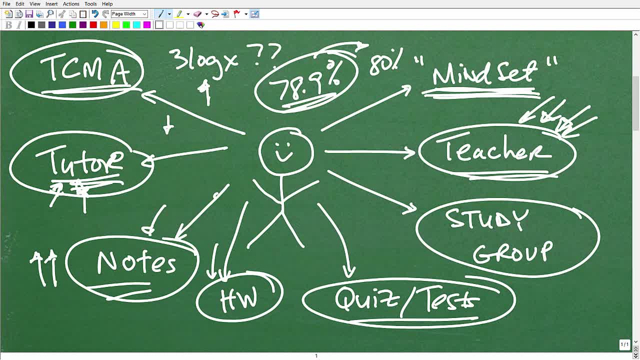 So that's why your attitude, your mindset, all This plays into a huge- you know it has a huge- impact on your overall grade. So, again, these aren't guarantees, but just being a teacher, knowing how most teachers are, 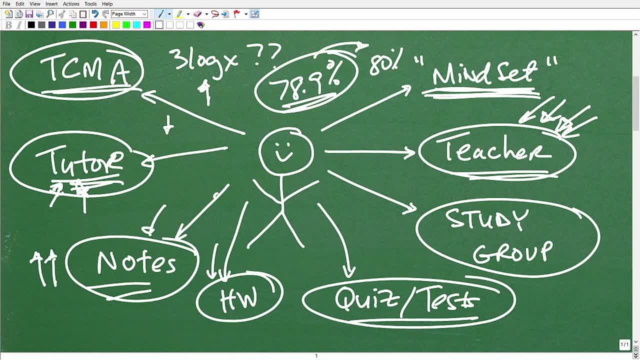 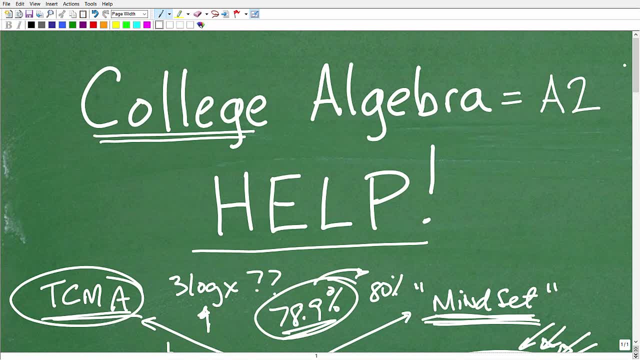 OK, these are. these are some really solid things that you need to kind of evaluate. Hey, where am I at with all this? Then you've got to be like: OK, college algebra, I'm just going to, just I'm going to do it.